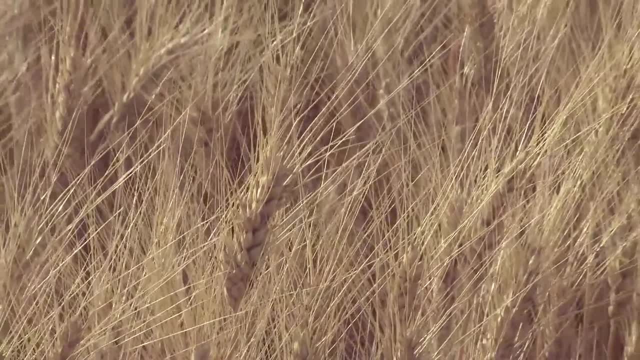 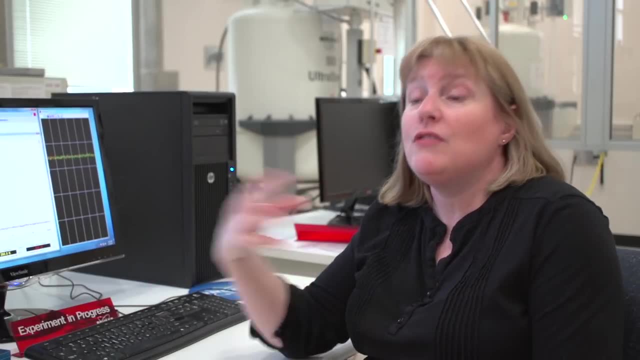 A lot of nutrient enrichment going back in from the grasses that were there, But as we start growing successive crops, we draw down our supplies of readily available phosphorus. We have a lot of phosphorus there. It's just not in the form that the plant can take up Phosphorus. 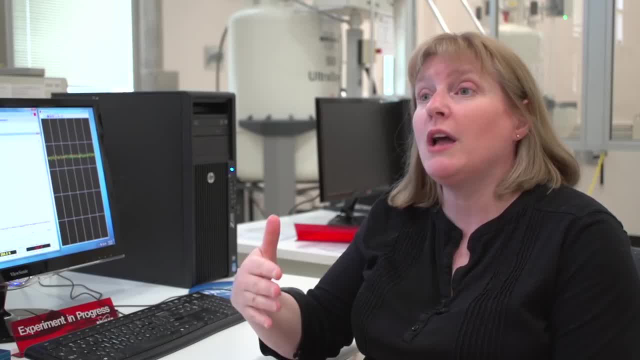 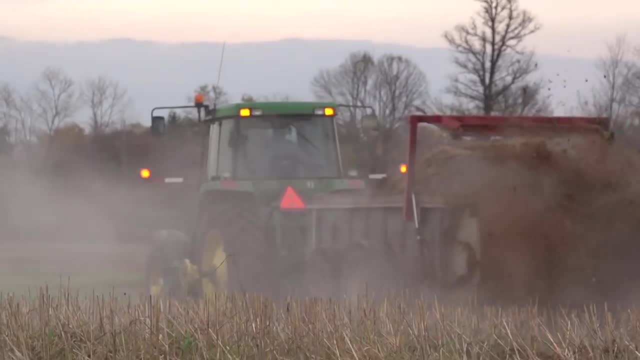 fertilizer is a limited resource because it's mined from rocks, And so we're going to run out of it at some point. what we need to do is start recapturing some of what is lost in waste from manure and human sewage sludge. Okay, we may not necessarily want to apply sludge. 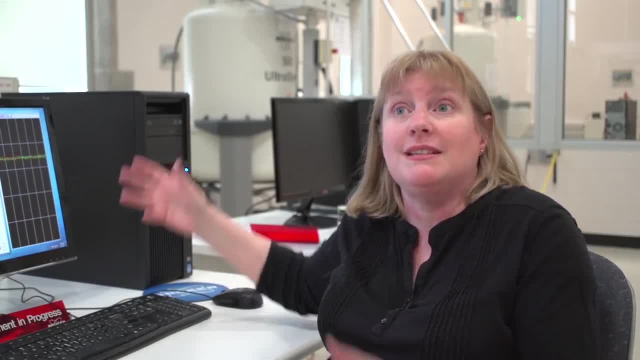 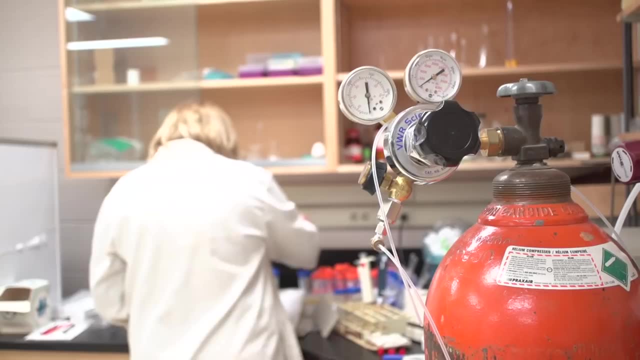 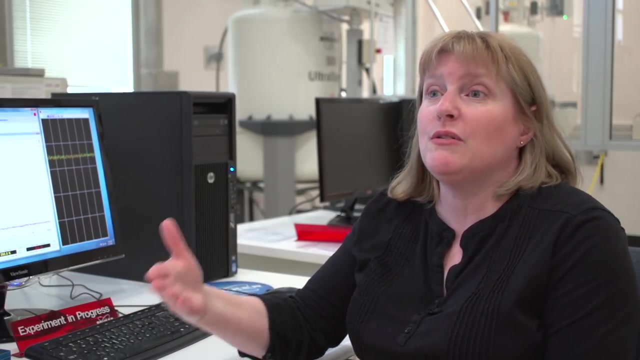 directly. but why can't we recapture that phosphorus chemically and find some way to convert that back into the fertilizer pellets that we know We can be much more strategic about what we apply but also explore other forms of phosphorus that are there and, you know, getting plants to use the native forms that are in the. 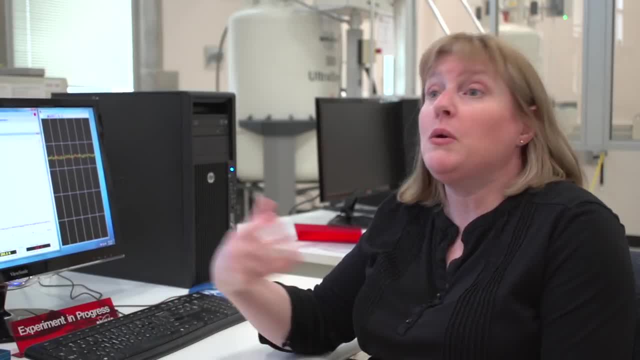 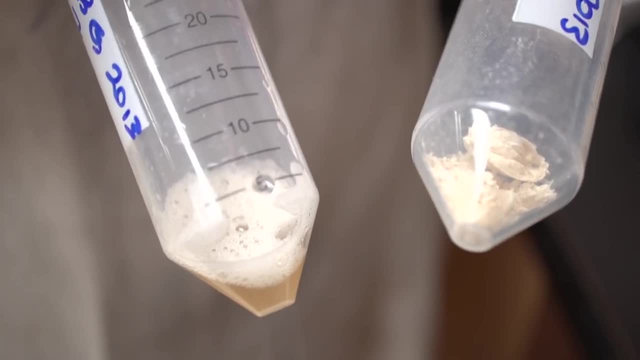 phosphorus rather than having to import something or microbes that may help the plants use it more. The development of nuclear magnetic resonance spectroscopy technology has allowed Agriculture and Agri-Food Canada scientists to understand phosphorus cycling at a molecular level By studying the cycle. 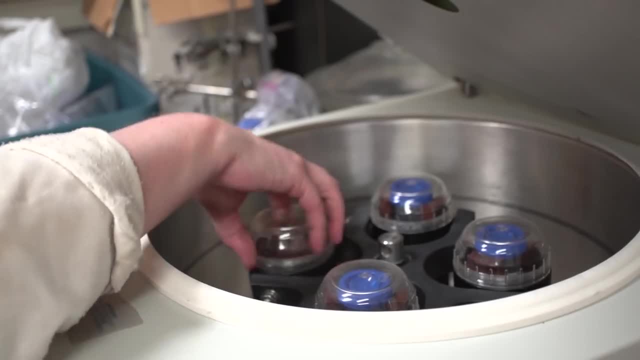 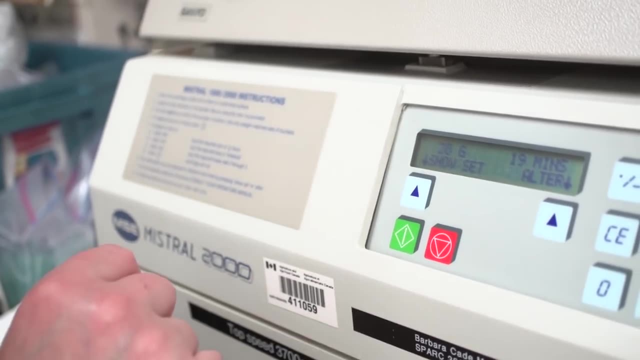 researchers get a complete picture of how phosphorus moves and thus get a better understanding of how to manage phosphorus more effectively. The goal is to make phosphorus fertilizer usage more efficient and environmentally friendly By reducing the amount of phosphorus lost each year from 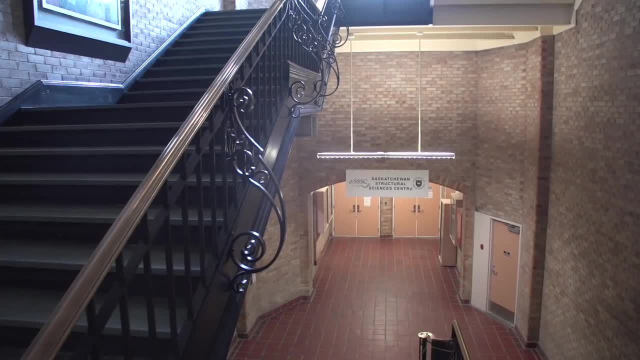 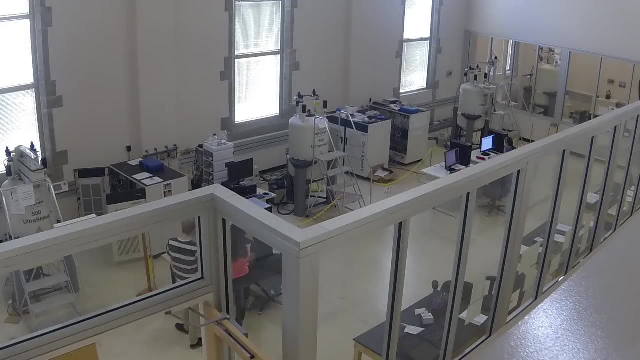 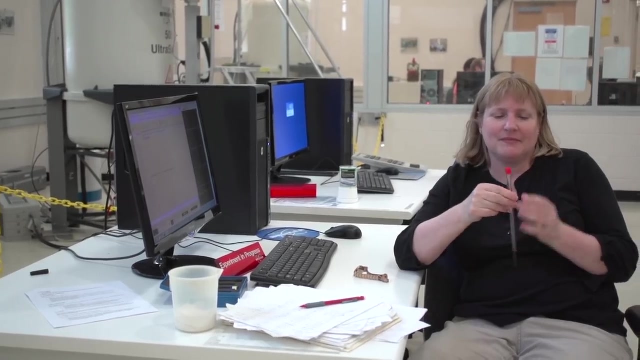 agricultural lands due to water runoff. This soil research is made possible by a partnership between AAFC and the Saskatchewan Structural Sciences Center at the University of Saskatchewan, With a probe purchased by the department. Dr Cade Menon uses the nuclear magnetic resonance machines at the University to 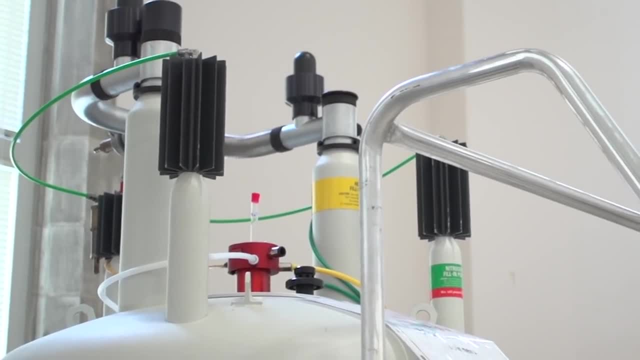 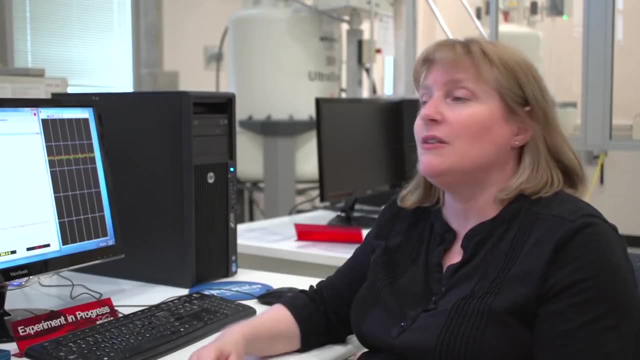 test her soil and runoff samples. We can take a sample and put it in a tube, so we're concentrating a lot of phosphorus. We put it in the soil and then we put it in the tube in that machine and that allows us to generate a spectrum which 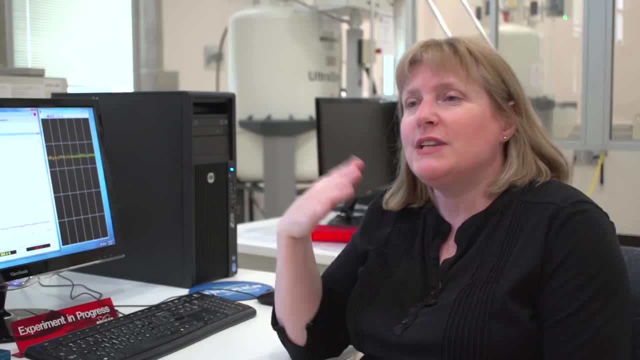 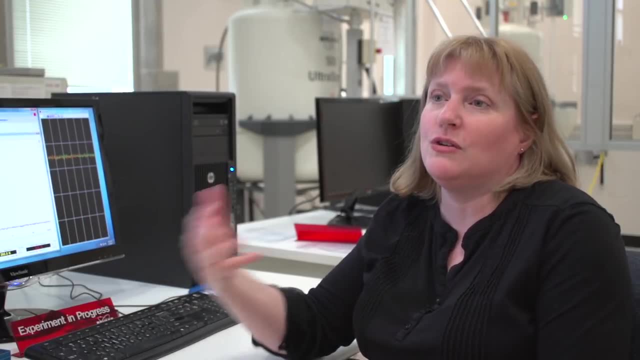 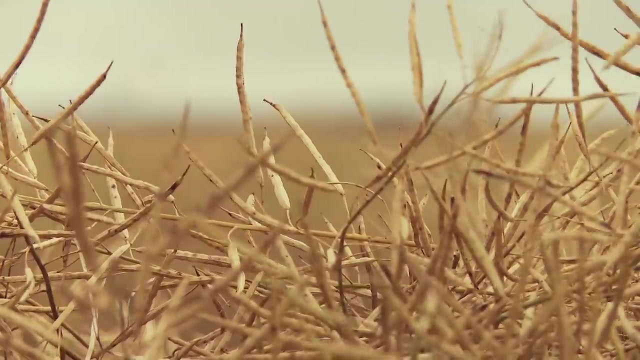 identifies the specific forms of phosphorus that are in there. The understanding ways to try to use exactly what we need in the form that we need it will help to make our fertilizer use more efficient. Knowing how to use phosphorus fertilizers more efficiently and understanding how a plant uses